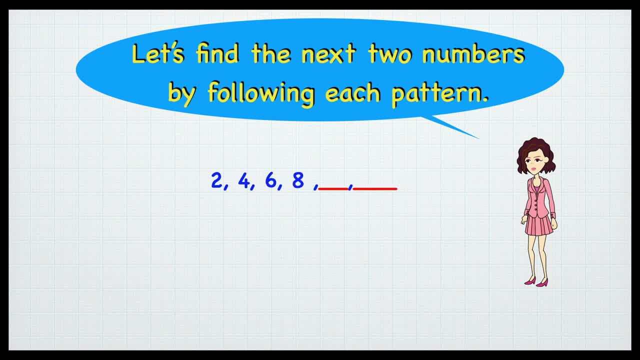 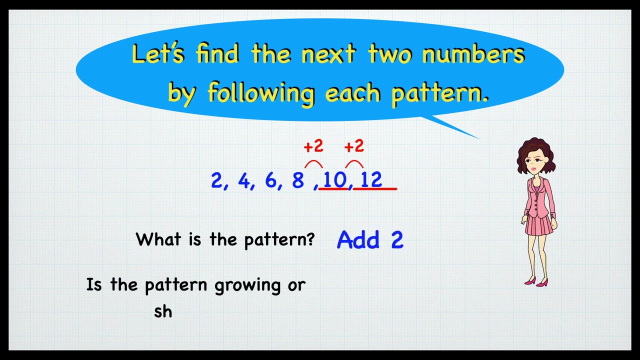 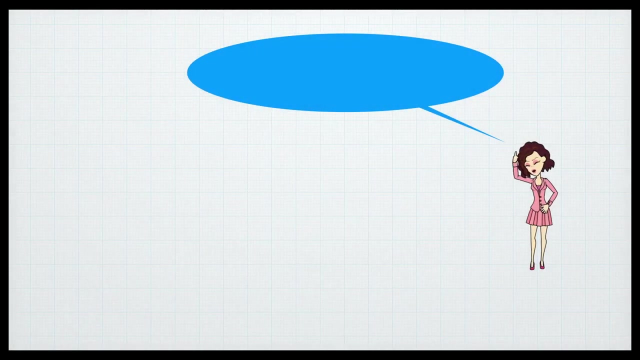 2, 4,, 6,, 8, 10, 12 plus 2 plus 2. What is the pattern? Add 2: Is the pattern growing or shrinking Growing? Let's try another one: 30,, 27,, 24,, 21. 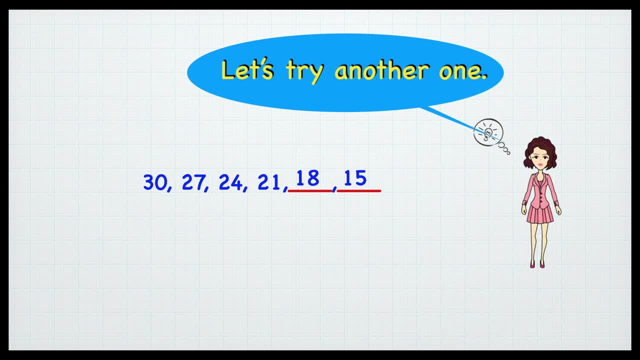 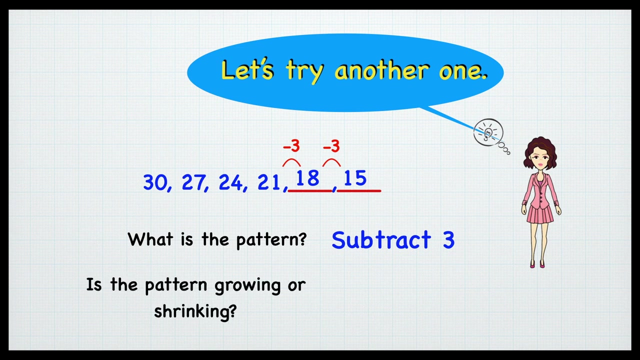 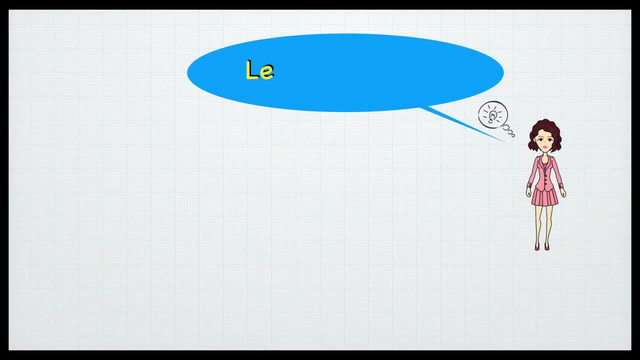 18, 15 minus 3 minus 3. What is the pattern? Subtract 3: Is the pattern growing or shrinking, Shrinking, Shrinking. Let's try this one: 0, 1, 0, 1, 0, 1. 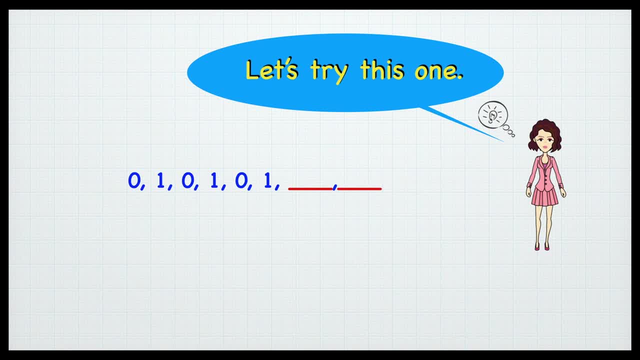 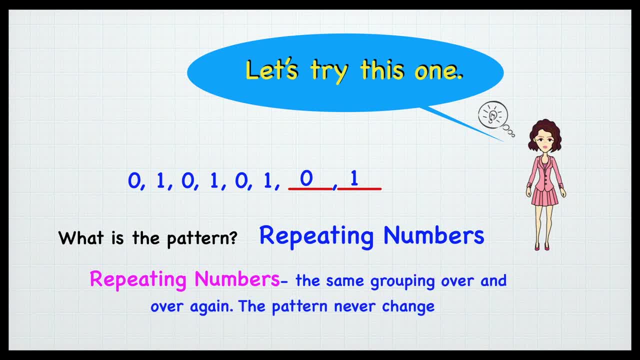 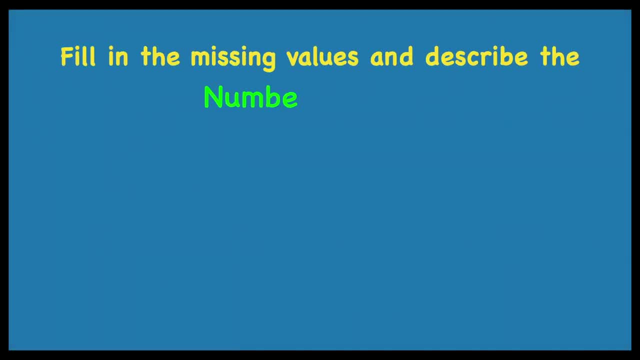 16,, 20,, 21,, 22,, 23,, 22,. never changes. Fill in the missing values and scrape the number pattern: 20,, 25,, 30,, 35,, 40,, 45.. What is the pattern? Add 5.. 25,, 22,, 19,. 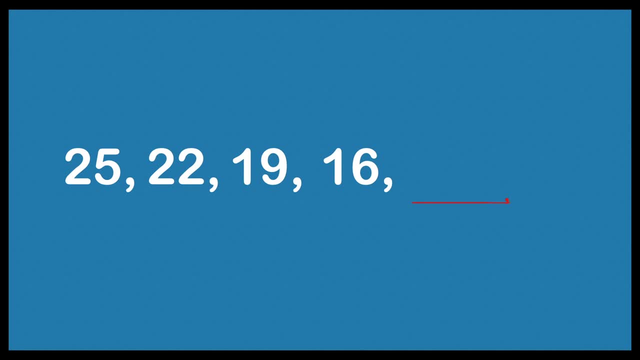 60., 16,, 13,, 10.. What is the pattern Subtract 3. 24,, 20,, 16,, 12,, 30., 8,, 4.. What is the pattern Subtract 4. 7,, 14,, 21,, 28,. 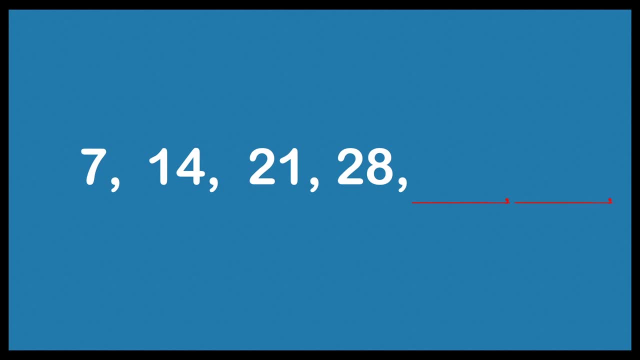 40, sauce, 46, 5,ixe Adobe, которые you're added to the index, 35, 42.. What is the pattern? Add 7.. 1, 2, 3.. 1, 2, 3.. 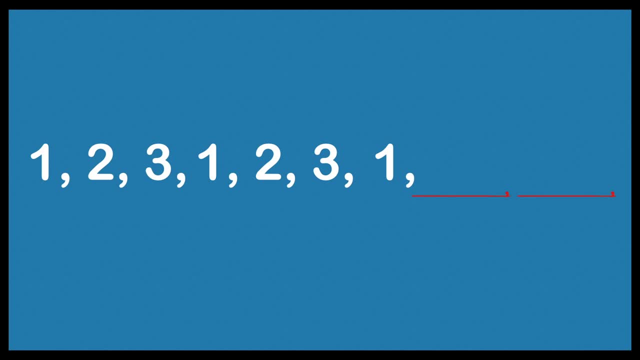 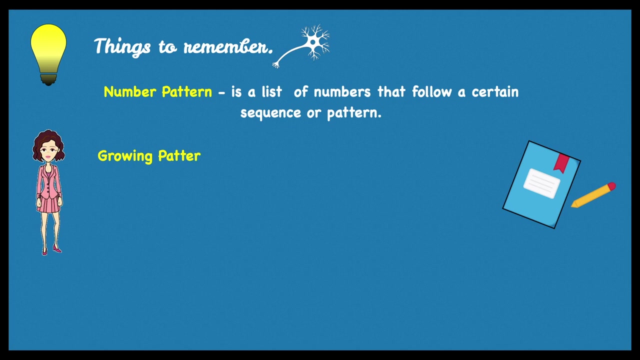 1, M, M, 2, 3, 7, 1, 1, 1, 3, 1, 1,, 2, 3. What is the pattern? Repeating numbers- Things to remember. Number pattern is a list of numbers that follow a certain sequence or pattern. 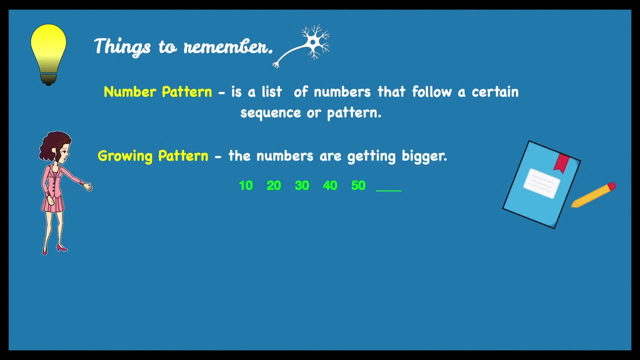 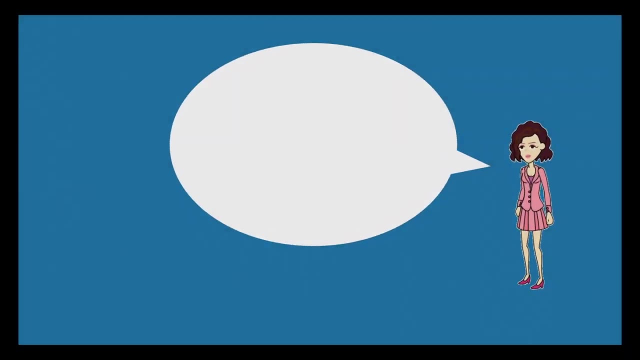 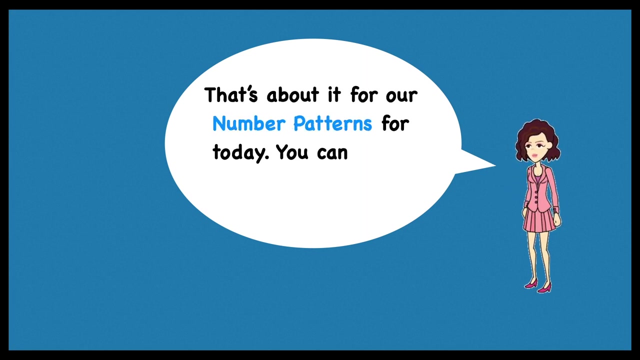 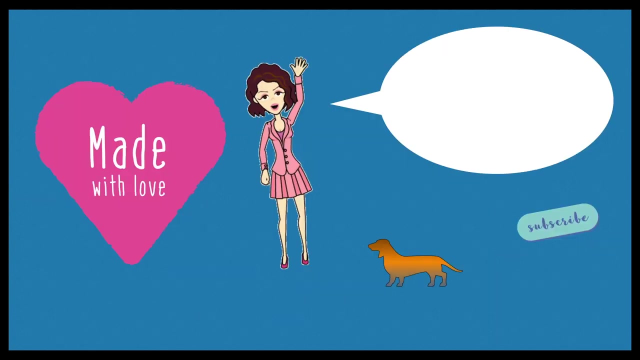 Growing when the numbers are getting bigger. Shrinking pattern. the numbers are getting smaller. Repeating pattern: same number grouping over and over again. That's about it for our number patterns for today. You can check my other videos about patterns. Thank you for watching. This is Aya saying bye, bye.